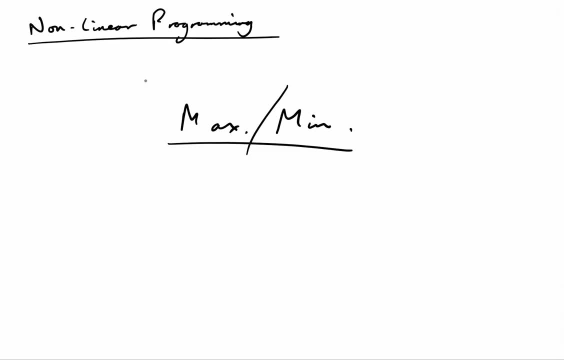 things, you know. time, for example, You know. this literally comes up all the time in everyday life. It's a very applicable way of doing things. It's effectively, you know, trying to find what the maximum or minimum way of doing things is. Now there is a word that is kind of linked to 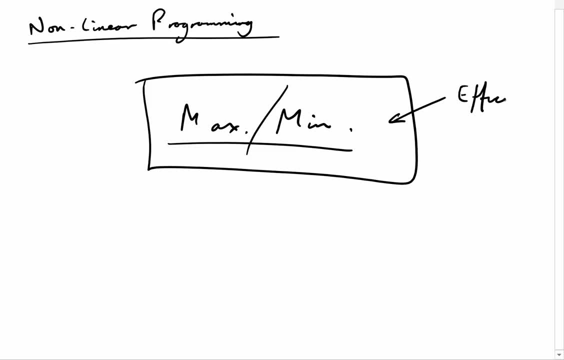 maximum and minimum, and this word is called efficiency. efficiency. Now, I'm loathe to use this word as such, because efficiency doesn't always mean the maximum or the minimum okay. So, for example, you could have something that is a maximum, So. 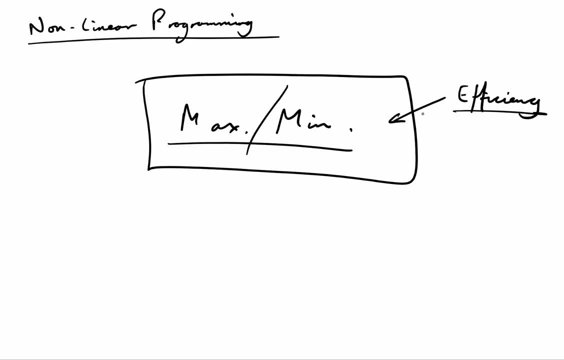 let's say, for example, if you have a supermarket chain that wants to work out the most efficient way of delivering goods, So if you're like you know, you've got supermarkets in, you know, represented by these dots and the chain here, okay, and these are all linked by sort of roads. 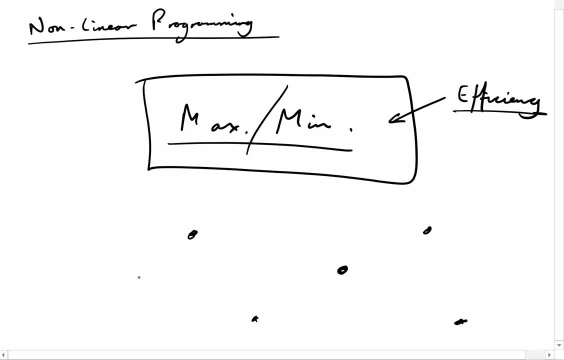 and motorways, and what have you? Yeah, okay, albeit this is a very simplified model, but hopefully you get the idea in your head. Well, the most efficient way of making a delivery may not always be the minimum way, So obviously you know you would have. 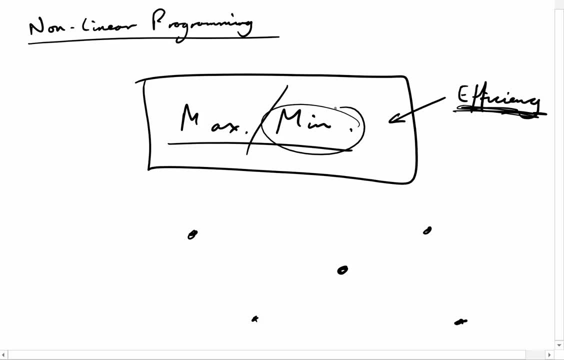 thought: oh, it would be the minimum distance which you cover. That may not always be the case, because there may be other factors which involve, such as time, for example. So the most direct route, in other words the route that takes the minimum distance, may not always be the most time. 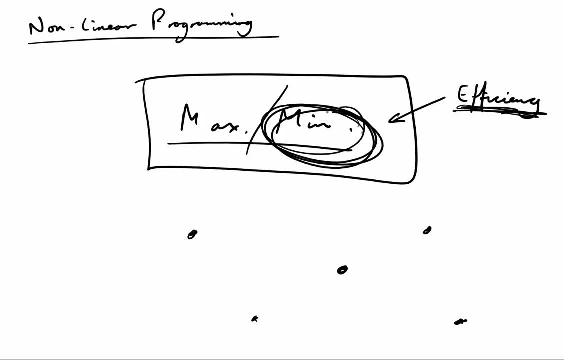 efficient route. You know, obviously using motorways will be a lot quicker than using all these back routes, okay, So you know, efficiency I'm kind of loathe to use. I'd much prefer you to use kind of understand a little bit more about maximum or minimum. So that's what we're going to. 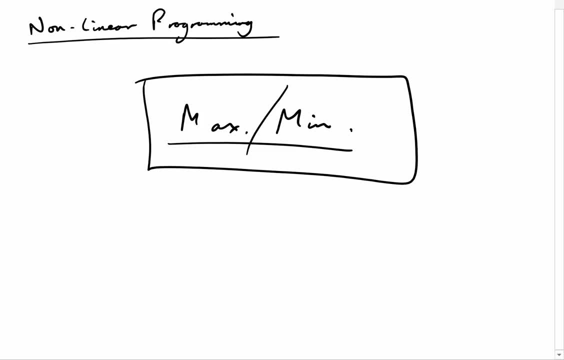 look at in this course. Now, there's two types of programming problems that we're going to look at. The first type that we're going to look at and we're going to spend sort of I don't know, I'd say a little bit more than half of the course looking at is the unconstrained problem. The unconstrained. 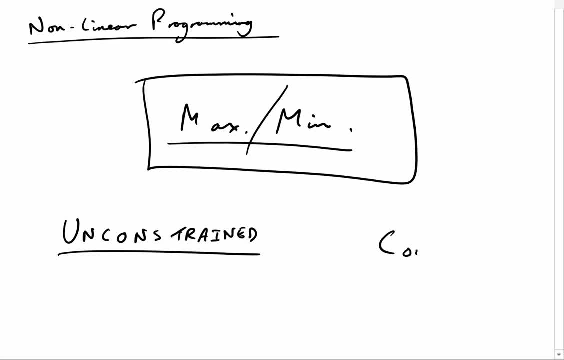 problem. So there's these things which are, you know, the other type. let me just write it down: the other type that we're going to look at are the constrained problems. okay, So you know we're going to spend a lot of time here and this is just going to build up the intuition a little. 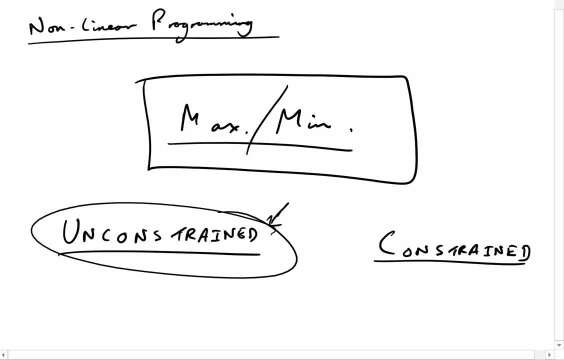 bit. So we're basically: it's more simplified. It's more simplified, but it may not be as applicable. So, you know, this is really actually. yeah, this is really. you know, this is really something that we're going to look at. Okay, so we will spend a lot of time here. All right, Now. 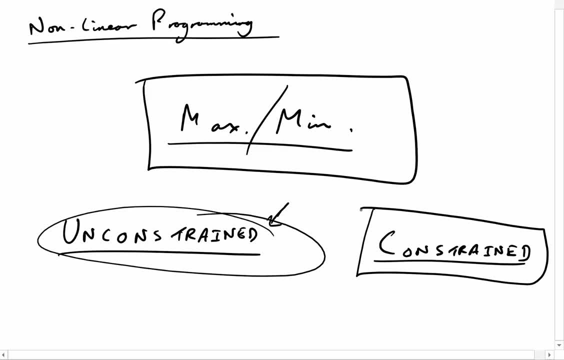 a constraint is basically a requirement that is needed. Okay, so a constraint is a requirement that's needed. So the first things first. it makes sense to start with the unconstrained problems because it's simpler, Okay, and it's slightly easier to sort of: you know, understand and get. 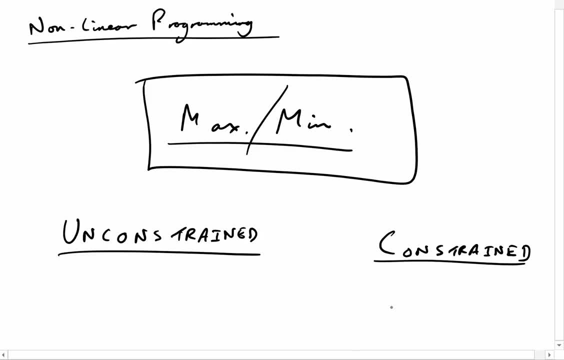 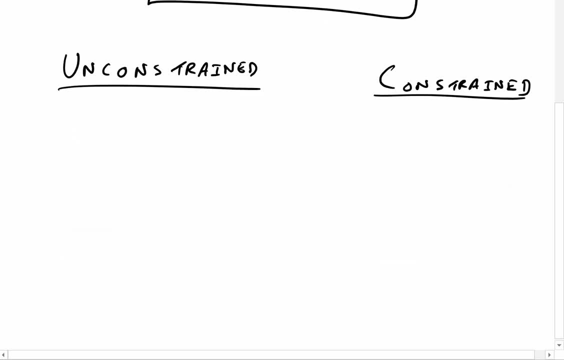 the intuition in your head. Okay, then, once we've got that intuition, you feel a little bit more comfortable and you know a little bit more familiar with it. then we're going to start looking at the constrained types. Okay, So let me just write out all the different methods that we're going to be looking at in this course. 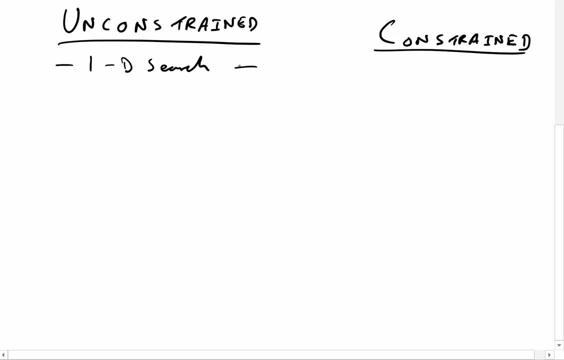 So the first type that we're going to be looking at is this thing called the one-dimensional search. Okay, Then the next type that we're going to be looking at are things like quadratic forms. Yeah, and hopefully you can kind of guess what that means, because you know the clue, there being 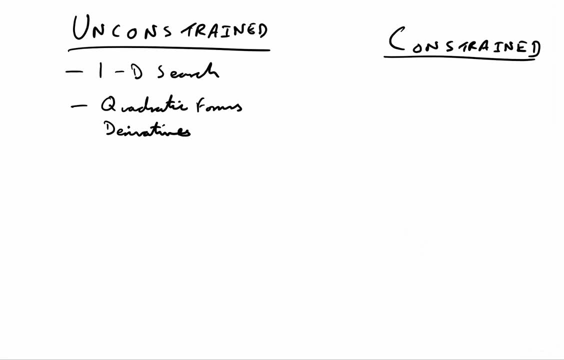 quadratic, so putting something into a quadratic form. Then we're going to look a little bit at derivatives. Okay, and associated with that is Taylor series. fairly obviously, when you want to find an approximation of a function in terms of its derivatives, Okay, and associated with that is. 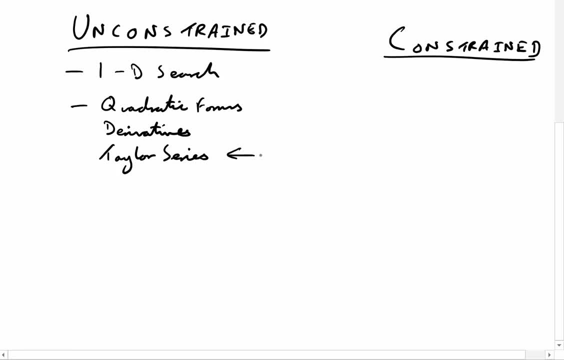 Taylor series. fairly obviously, when you want to find an approximation of a function in terms of its derivatives, It's known as the Taylor series. so you can use the Taylor series to do that, And also we're going to look then at, so the types of conditions that we have to impose for maximum. 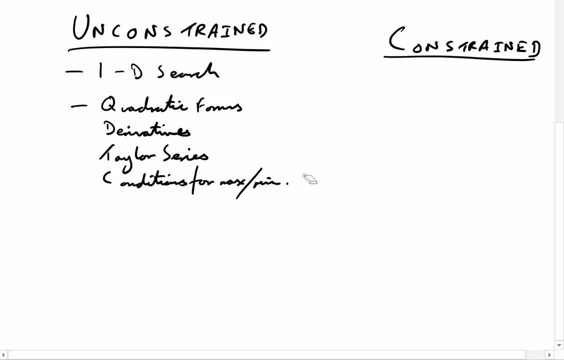 and minimum requirements. Okay, Then we're also going to look at this thing called gradient search, right, which basically you know you can, hopefully you can see you've got search there, So you've got a one-dimensional search here and you've got gradient search down here. Then we're 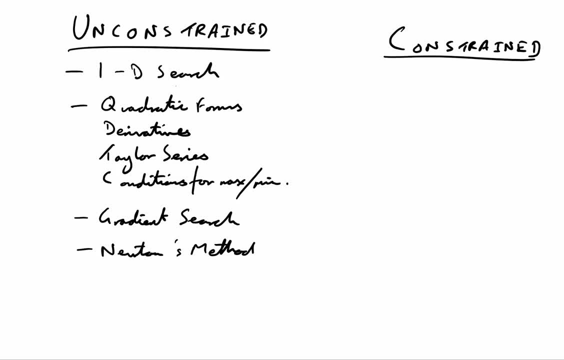 going to look at another method, which is Newton's method. So this is another search method that we tend to call gradient search. So this is a, you know, a gradient search method. So this is a method, And the last type for unconstrained problems is the is the quasi-Newton method. So 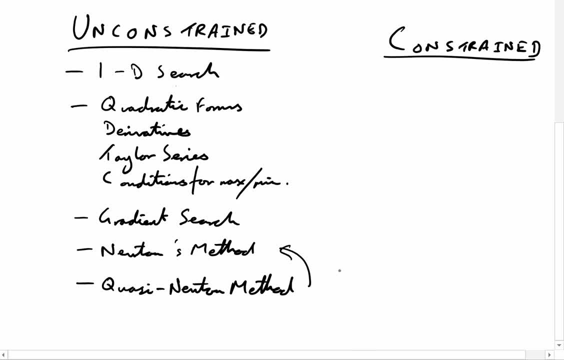 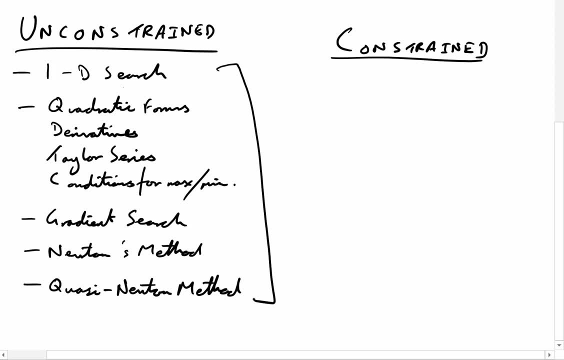 it's a little bit more advanced than Newton. We kind of identify some problems in here and we basically, you know, correct them in here. So then let's come on to the constrained problem. So these are all the types of things that we're going to look at in the unconstrained things. Okay, then 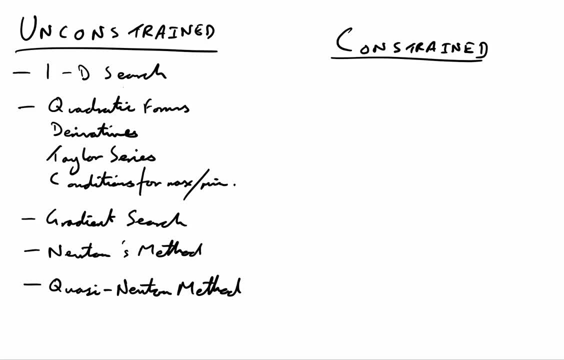 we're going to come on to the constrained problems And the first thing which we're going to look at. well, there's two types of constraints, Okay, There's first of all, equality constraints, So, in other words, a constraint which has you know, a constraint which has you know, a constraint. 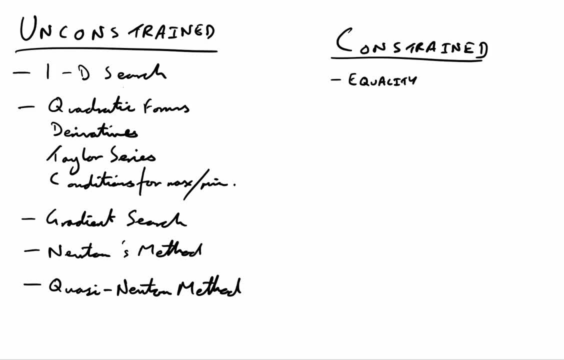 which has an equality, basically saying that we want something equal to something else. So, for example, we could have- we want a requirement that we need to make exactly three, three types of one product, for example. So the number of products that we have to make would be three. So that would. 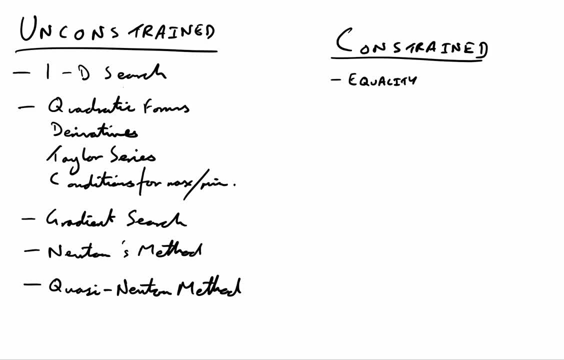 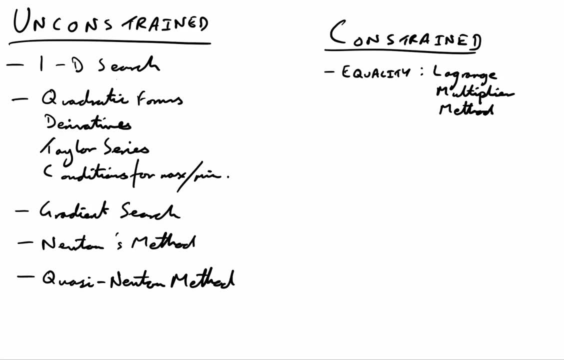 be an equality constraint And coming under. you know the type of method that we use is for equality constraints, the Lagrange multiplier method. Now, many of you may have met that before in you know, in mathematical methods, But we'll go over it again anyway and we'll look at it in a slightly different way. And the other 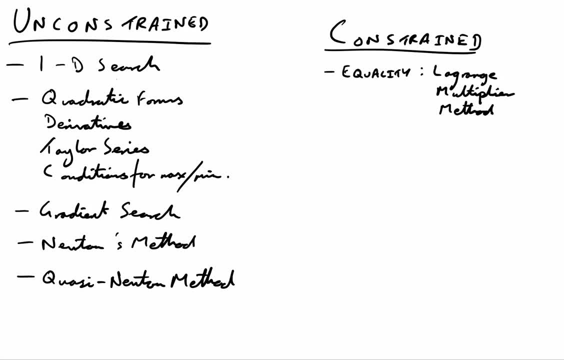 type, of course, if we've got an equality constraint. so in other words, when you you know we've got an equals sign, so an exact, if you like, then the other type would be where we can have exactly so. 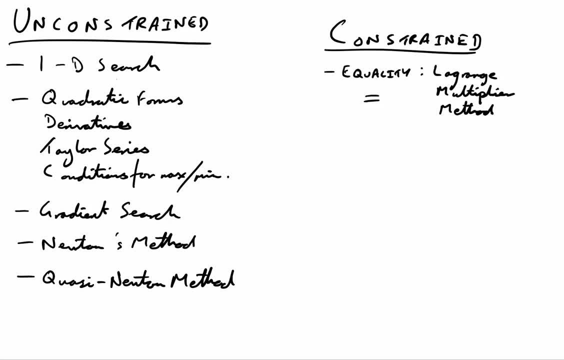 more than or less than, for example, And these are what is known as inequality constraints. So, likewise, you know, we can have less than something or greater than something. So we're basically saying that we need to make at least three types of one product, or we have to, or 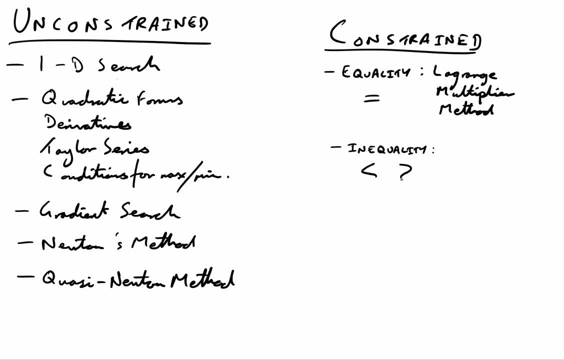 for example, there might be a requirement on work staff or the staff that make the work. So we have to basically say that you know we cannot make more than this amount of one product, for example. So you know there's many options where an inequality constraint will come in. 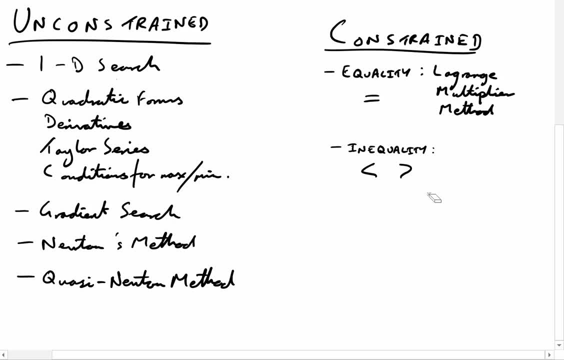 Right, And we'll talk about how we talked about in linear programming, how we can convert an inequality constraint into an equality constraint by adding some what's known as slack and surplus variables, So in other words, some amount that we have to add to to make it into an equal equality. 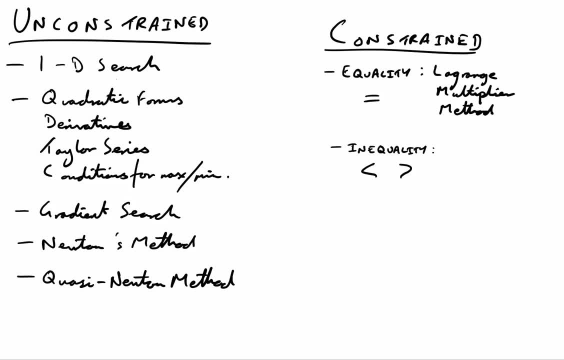 Apologies about that. So let's, let's talk about then, so the types of- you know the types of things that we look at with inequality, is this thing called the, is the KKT conditions, And KKT stands for one minute, Karish Kuntaka conditions, but we tend to just abbreviate it to KKT. Okay, And the last thing that we're going to look at in constrained problems and constrained, constrained programming, is this thing called penalty methods. 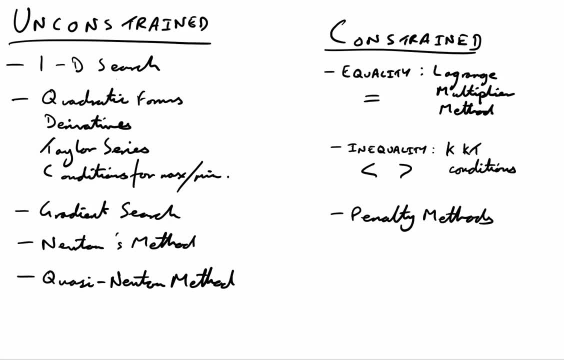 So, in other words, if we do something, then there's a penalty which is associated with it, And so we're going to kind of look at methods, methods that deal with that- to basically make the most efficiency. So this is this is where efficiency very much comes in. You know, we want the most, we want the most efficient way of doing things. Well, sometimes that comes at a cost, And we look at that in this part there. 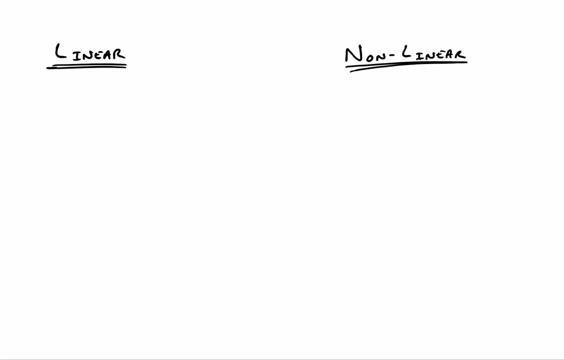 So, okay, what is the difference, then, between a linear programming problem and a nonlinear programming problem? We tend to abbreviate linear programming problems As an LP- okay, and a nonlinear programming problem as an NLP- Okay, and we tend to spend the majority of the time in this course. I mean, this was in another module, So we tend to spend a majority of time in this course. But what's the difference between the two? What's the difference between the two? Well, for a start, linear programming problems tend to be slightly more straightforward to deal with. Okay, there's, there's various methods that can be used to sort out nonlinear sort of sort out linear programming problems. And again, you know, you're probably familiar with these. I mean, you met a lot of them at A level. You met a lot of these methods at A level. 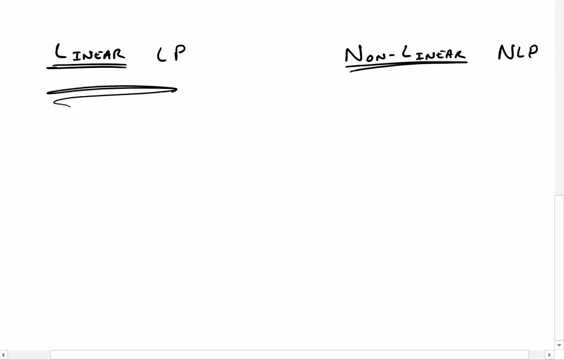 Which is kind of a good indication that they're not actually that tricky. They can be tricky, but they're not. they're slightly. the ideas behind them are slightly more straightforward, Whereas these nonlinear problems, nonlinear programming problems, come up an awful lot more in the real world. 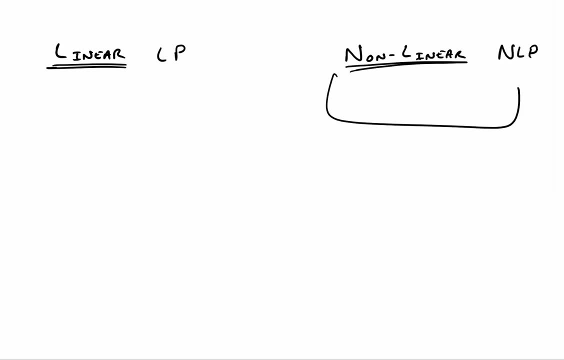 Because, as you probably guessed by now, very few things in the world have a linear relationship. So in other words, as one thing changes, the other thing changes by a proportional amount, sort of a multiple. There's usually kind of other more advanced functions. 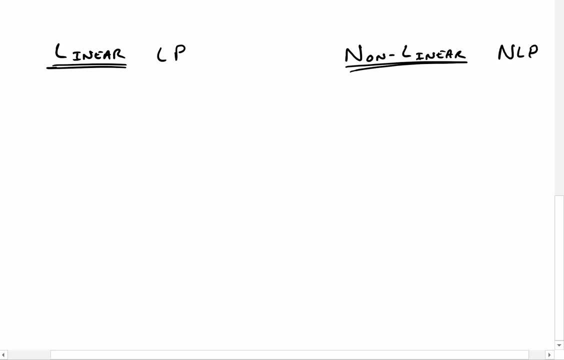 Which are going on, another more far advanced relationship between things. So it tends to be kind of more like curves rather than a straight line. Yeah, that's the relationship between things. So what's the difference between a linear programming problem and a nonlinear programming problem? 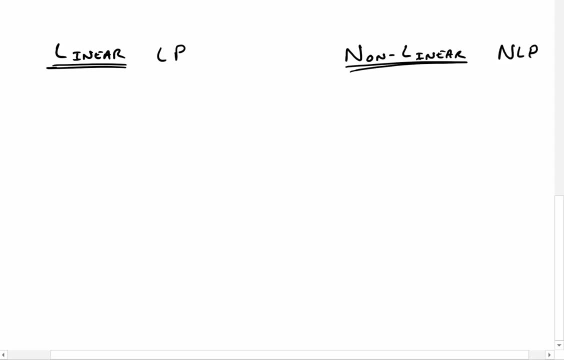 Well, a linear problem, a linear programming problem, is usually where the unit price is fixed, or the distance or whatever. It's normally where it's fixed. Okay, so, in other words, it can't change. So, for example, if we have two variables, x1 and x2,, x1 and x2.. 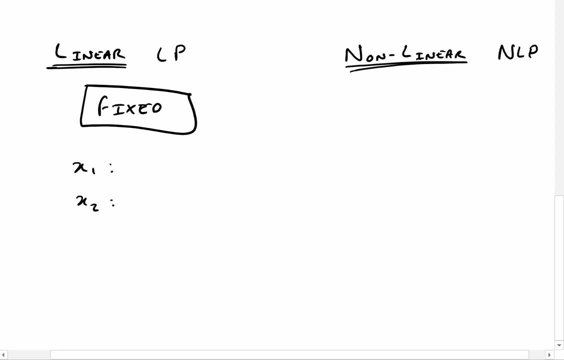 Now, these could be anything. you know, these could be anything from Products to so this is one product and this is another product, for example, This could be one supermarket and another supermarket, for example. Yeah, they're just, they're just variables, basically. 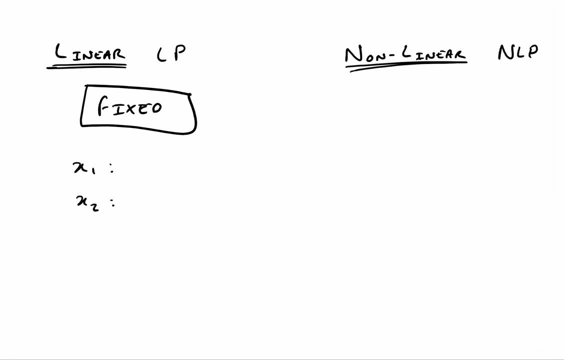 So, for example, for a linear programming problem, say, for example, if we're dealing with price, x1 might be 14 pounds and x2 might be 20 pounds. Okay, so it tends to be where the, where the price, where it's fixed. 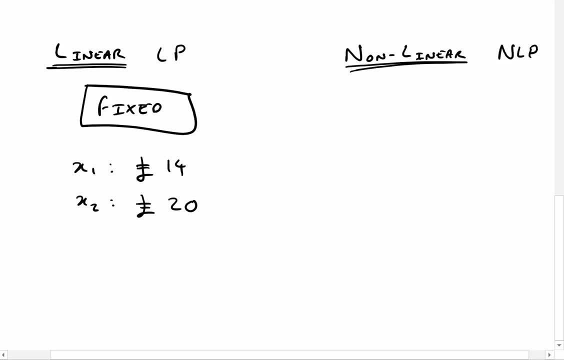 Okay, whereas with a nonlinear programming problem it's not fixed. So, in other words, it varies. it varies, Okay, oops, varies. So that's the idea with a nonlinear programming problem And quite a lot of the time it's given in terms of the other variable. 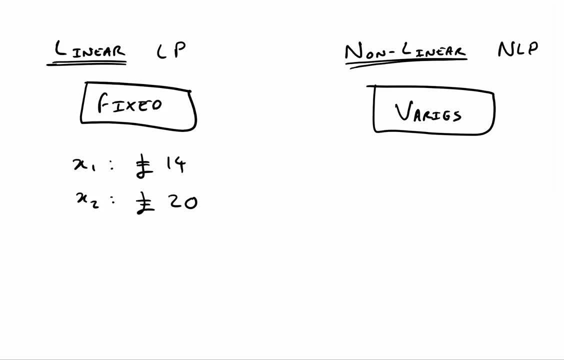 So it depends on what the other variable is doing. So, for example, if you're talking in terms of price, then x1, x1 might be given as or yes, or let's say let's yeah, okay, let's stick it with price. 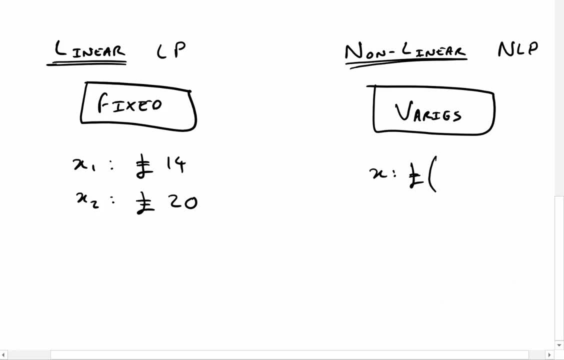 Because it doesn't really matter, it's just being made up. So let's say that x1 is given in terms of what x2 is doing. So maybe price- Price isn't the best example, but maybe you know number of units which are made. 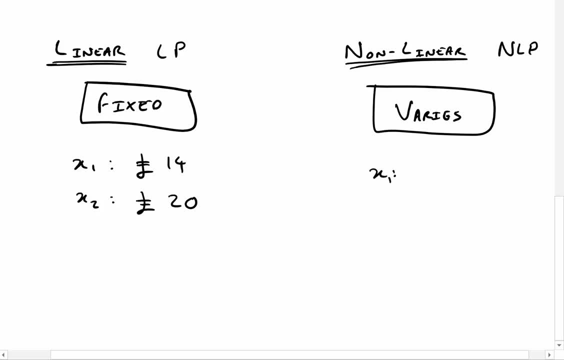 Let's say number of units which are made. you know x1,. the number of units of x1 depend on the number of units for x2.. For example, x2 might be another component which needs to be made in order to make x1. 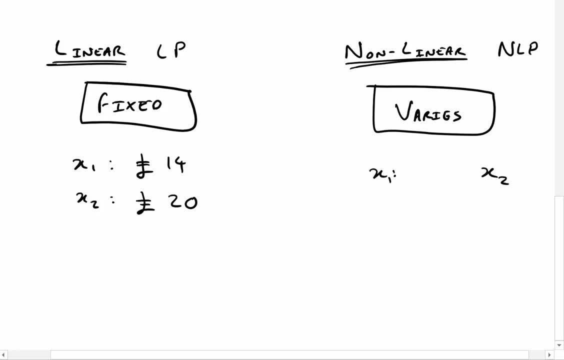 So you know, we need to make so many amounts of x2 in order to in order to make x1. So, for example, you know this might be 7 minus 3x2.. Yes, x1 might be given as 7 minus 3x2.. 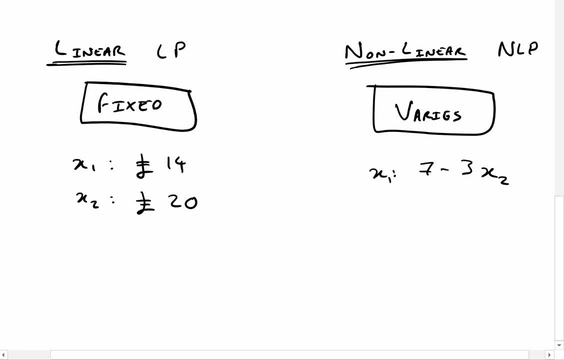 So that's the idea behind nonlinear, Nonlinear and linear problem. Basically linear problem, we tend to have fixed, we tend to have fixed values. Okay, so the unit price is fixed, Whereas or the unit distance or whatever, Whereas with nonlinear problems tends to be ones given in terms of the other. 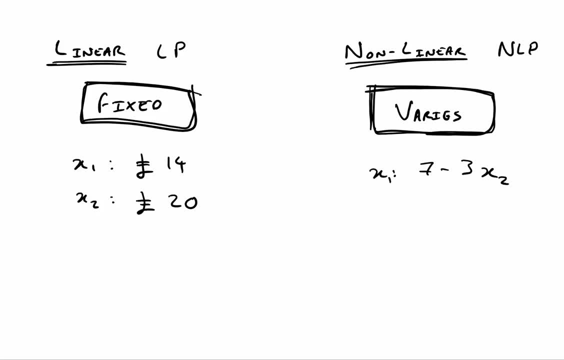 Or at least it varies. So it varies by some amount. Right Now, the method behind how we set up a nonlinear programming problem and a linear programming problem is exactly the same. So how do we set it up? Well, the first step, the first step, is always to define your variables. 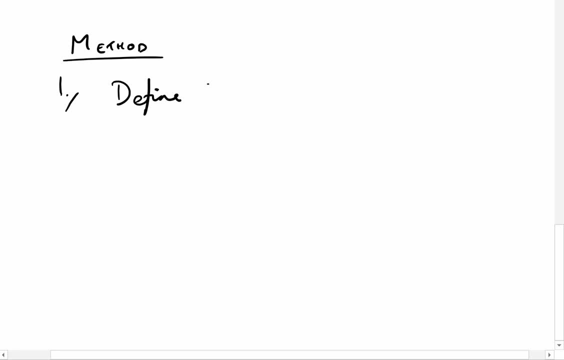 Okay, What do you have? You know, oops, define variables. Okay, So you know, say, for example, if you have x1. So you have products, you know you want to define x1, x2, and so on and so on. 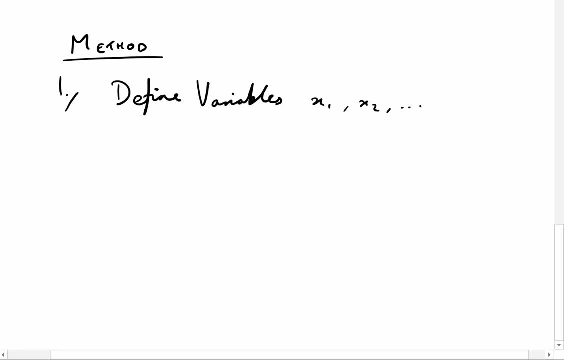 Notice that we tend to define it sort of using the same letters. So normally you define it using, you know, usual methods like define it as x1, x, y and z, for example. Well, the trouble is with defining it like this is that we've only got a finite amount of letters. 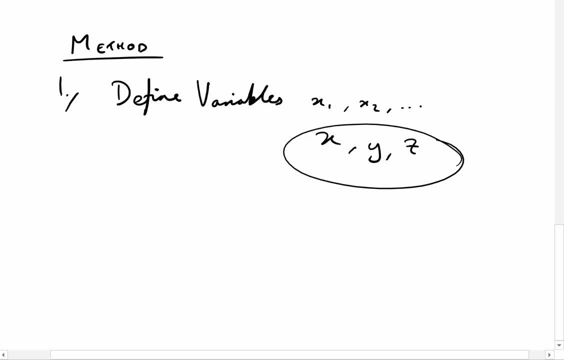 And theoretically you could have a programming problem. And with hundreds of variables going on, hundreds of variables going on, For example, I'm thinking shipping of container ships. Okay, If you go down to the docks you've got literally hundreds of container ships. 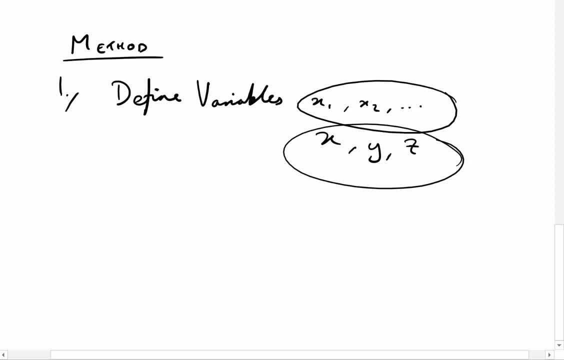 Well, you want to define each container ship with a variable? Yeah Well, fairly obviously, there's going to be more than 26 variables, And I say 26 because of course, we've only got 26 letters available to us if we don't include Greek letters or whatever other letter alphabets. 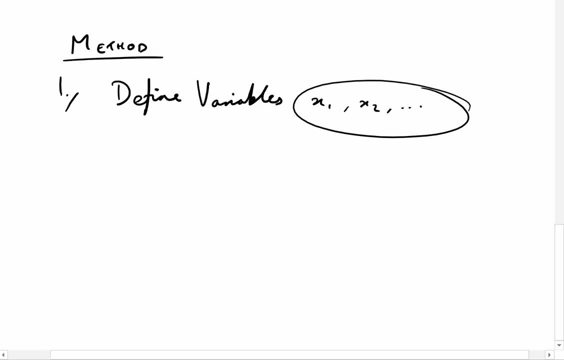 So we tend to write it like this, So we tend to say, right, Okay, X is our variable, So let's say X with some subscript, So we call it XI. Okay, It's just basically say, for example, container ships. 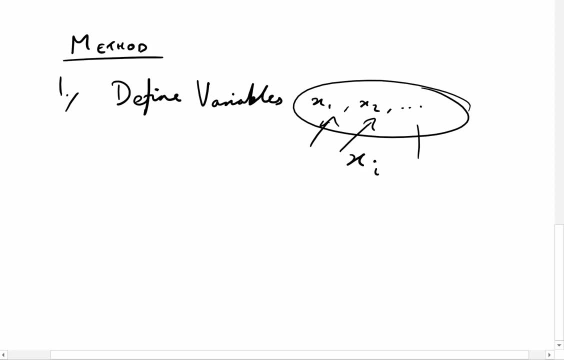 Okay, And this is our first container ship, This is our second container ship And we can carry on going right through. Okay. So this is why we tend to define it using this subscript notation, And we tend to always do that Right. 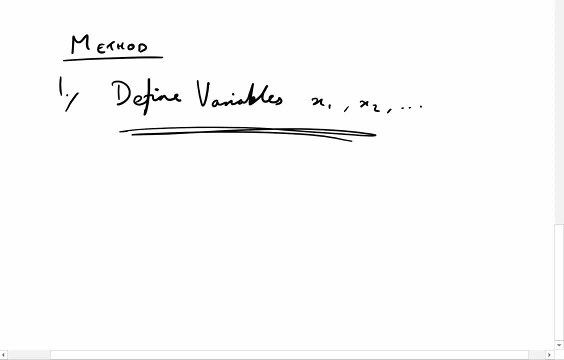 So that's our first step. You know, we want to define our variables, We want to look and see what we're actually working with. We want to look and see what we're actually dealing with. The second method then, or the second step: 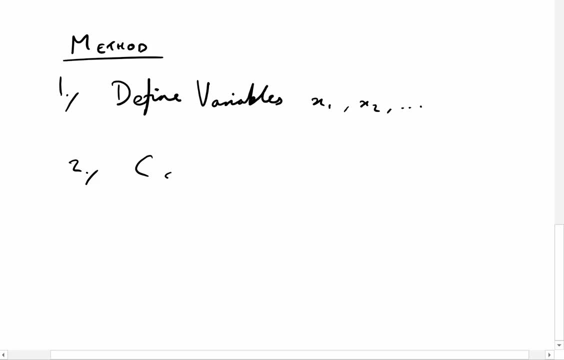 The third step is then to define our constraints. Okay, Define our constraints. So basically, you know, are there any requirements that are needed? You know. so another word for restraints are requirements. Okay, So basically, you know, you need to say: are there any requirements that need to be satisfied before you know for our problem? 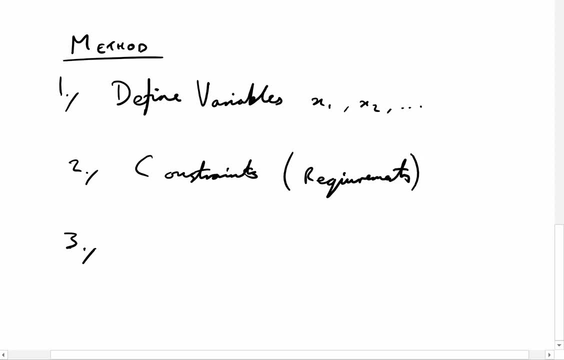 Right. And the third step? the third step is then to form the objective function. Of course the fourth step is implied. Fourth step is then to go ahead and solve it. But this is just setting up The penalty, the programming problem. 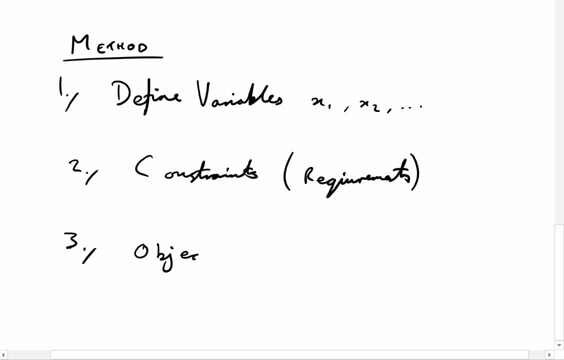 So the next step, then, is to set up, or to define what the objective function is. What the objective function is Okay. So, in other words, do we have to- and that also includes whether we have to maximise it or whether we're looking at a minimisation problem. 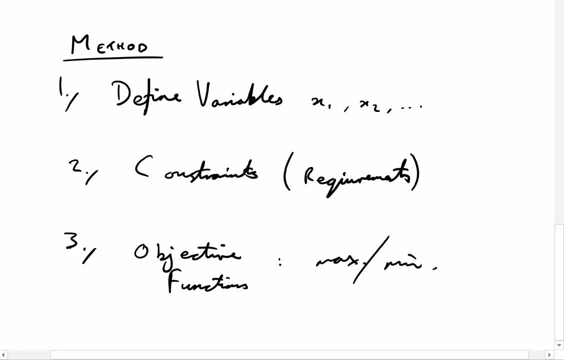 So we're only going to be looking at either a maximise or a minimise. We want to get the most out of it or we want to get the least out of it. So, for example, cost is normally to do with minimising. 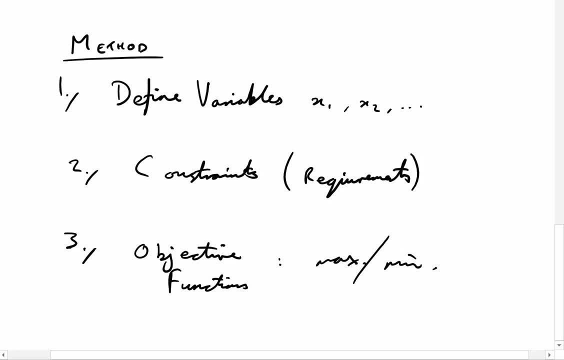 Yeah, So maximise or minimise, basically Okay, Okay. And the main types, the main types of objective functions. So, for example, we could be dealing with cost. So cost is normally given by, so we'll have price per unit. 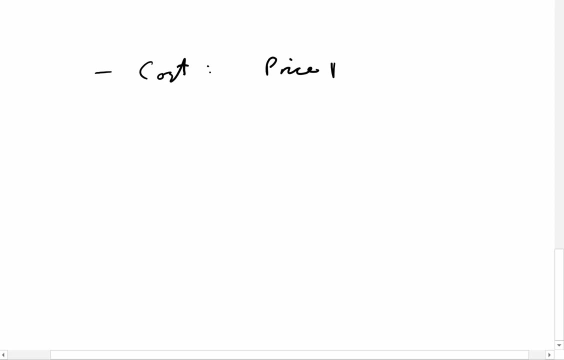 Okay, We'll have price per unit. So, for example, price per unit. So, for example, we might say: it costs three pounds to make X1 and four pounds to make X2.. So three pounds for X1.. So this is our first. 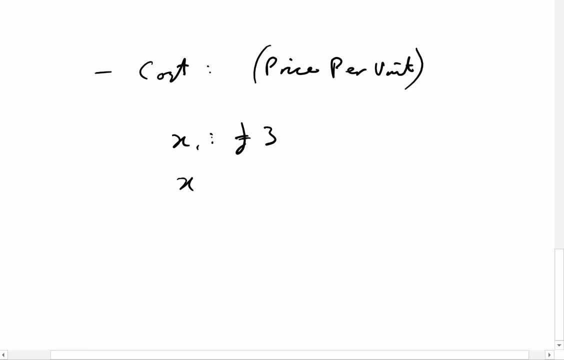 You know, X1 is our first product, X2 is our second product, And it might cost four pounds to make X2.. Okay, But then we need to multiply it by the number of units that we make, So the number of units that we end up making. 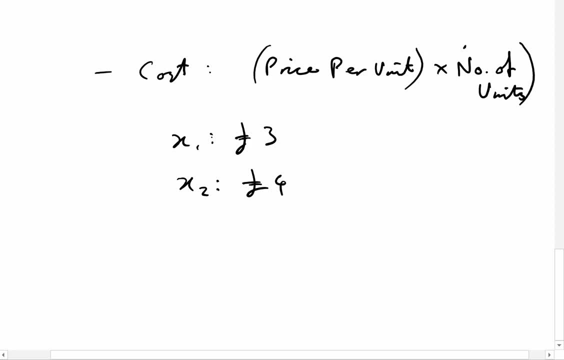 Number of units. So, for example, I always think of the objective function, The objective function, I always think of the objective function as, if you like, the total. That's the thing that we want to get. You know, that's the thing overall. 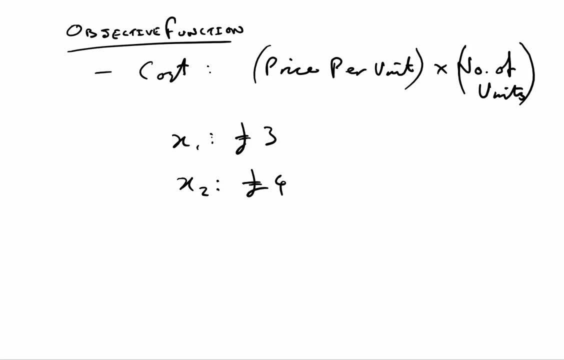 So we've not broken it down, We've got to put everything together And this is almost like the total. The objective function is almost like the total. Okay, So cost is price per unit times number of units. So let's say, for example, you know, X1 costs three pounds to make. 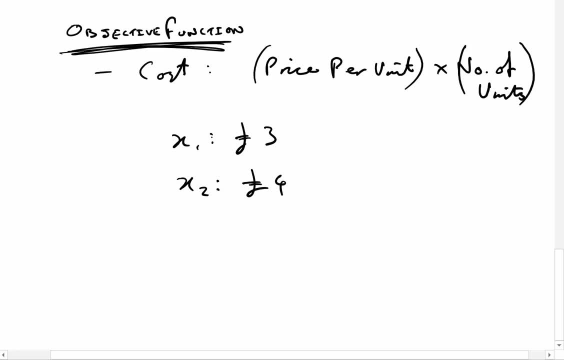 Each unit of X2 costs four pounds to make. So this is price per unit, right? And let's say we make three units of X1 and six units of X2.. Well, what is our total? Well, it'll be three lots of X1 plus what did I say? 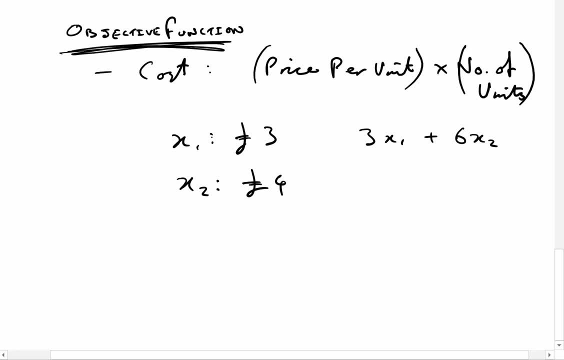 What did I say? Six lots of X2.. I can't remember exactly what I said: Three lots of X1 we make And six lots of X2.. So this would be our objective function okay, And we normally denote it by Z. 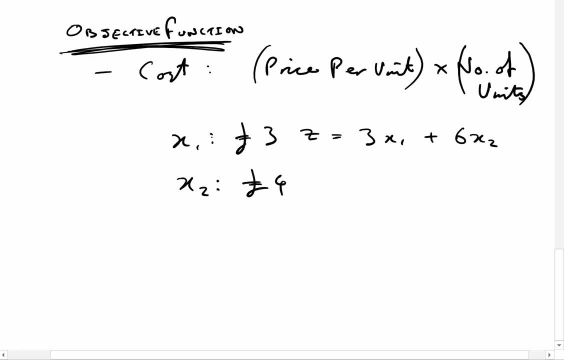 And so that would obviously be. we want to minimize or maximize that, okay, for example, Another common example of an objective function is time. So we could have time, Similar kind of thing, you know, similar kind of thing. We set up a similar kind of way to this up here.